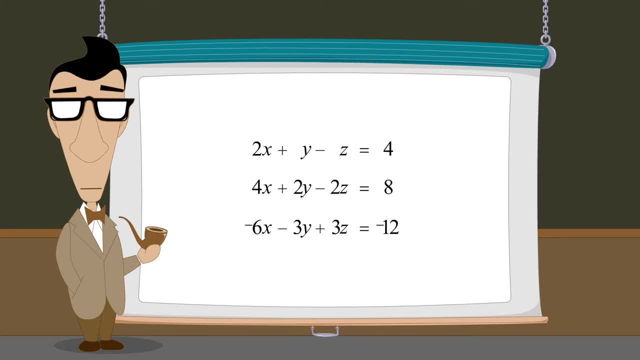 each other will describe the same plane. Therefore, if the equations in the system can all be made identical by multiplying by constants, they all describe the same plane. In this case, the solution set of the system is described by any of the equations. However, when all the planes intersect along a line, 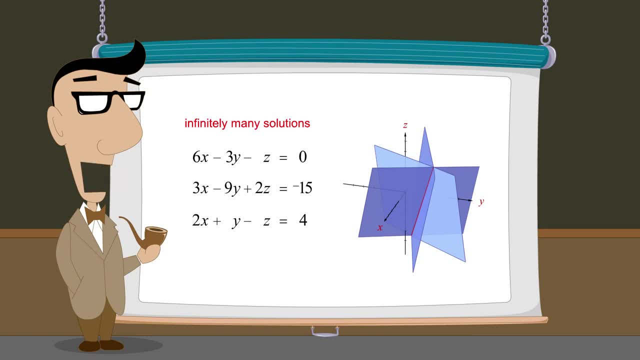 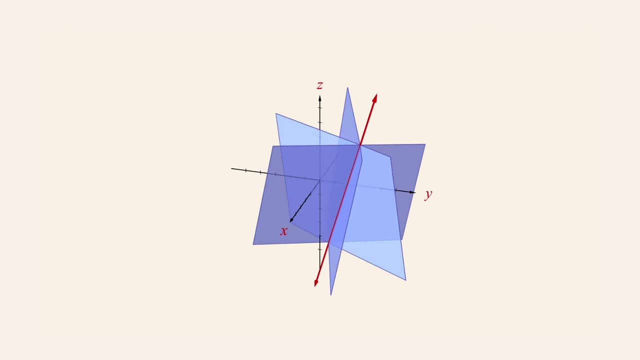 then this solution set is not described by any of the equations. We need some other way to describe a solution set whose graph is a line in three-dimensional space. Since a line in three dimensions is a linear object, you might think that it could be described by a linear equation in x, y and z. 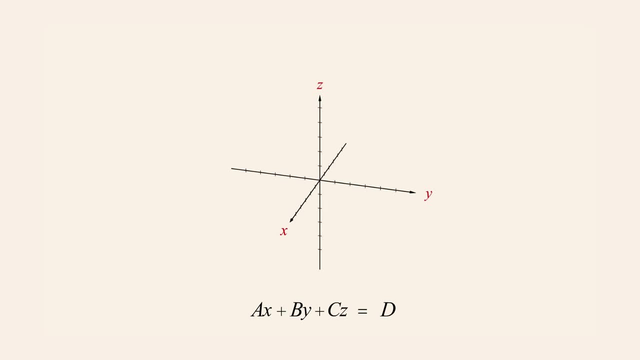 But, as we have seen, linear equations are not linear. Linear equations in three variables describe planes, not lines. In order to mathematically describe a line in three-dimensional space, we need a way to define the values of the three coordinates at every point along the line. 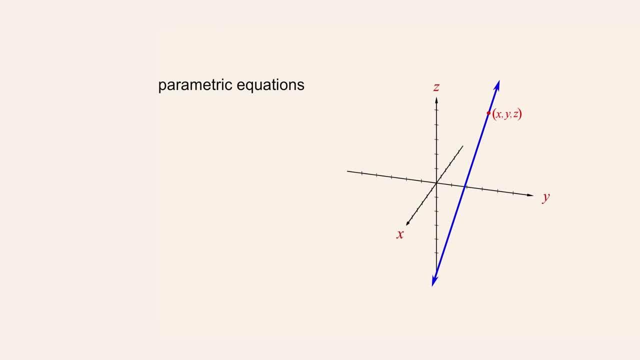 This can be done by creating a group of parametric equations, one equation for each of the three coordinates. Each parametric equation expresses the values of the three coordinates. Each parametric equation expresses the values of the three coordinates as a function of an additional variable called a parameter. 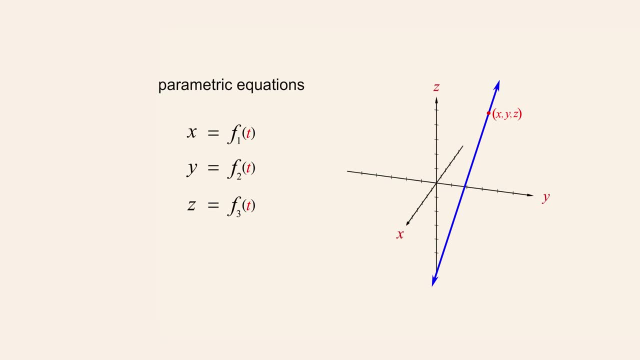 In this example, we have chosen the letter t to represent this parameter. For any given value of t, each of the three parametric equations determines a corresponding value for one of the three coordinates. For example, the values of x, y and z could be equal to t. 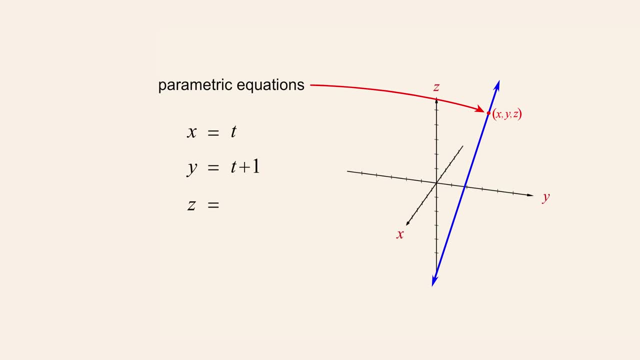 t plus one and three t minus three. So each value of t corresponds to an ordered triple which describes the position of one point on the line. In a parametric equation, the parameter varies freely over some defined range of values, Since in this example,